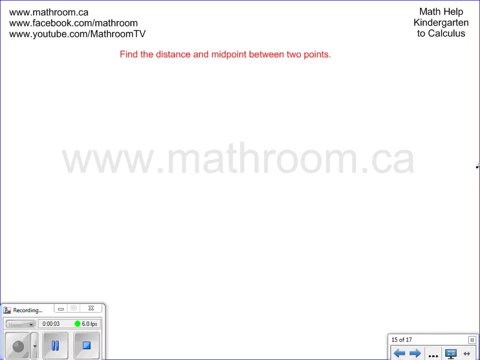 Okay, this time we're going to find the distance and midpoint between two points. Let's say we're given the points minus 2, 3, and 3 minus 9.. First of all, the distance formula is x2 minus x1 squared, plus y2 minus y1 squared, and we're going to take the square root of. 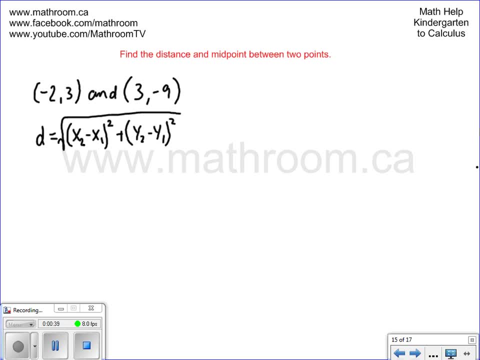 that number. First of all, we'll assign x1 and x2.. This is point number one. so we'll go x1, y1, and this will be x2, y2.. And now let's plug in those numbers into the distance. 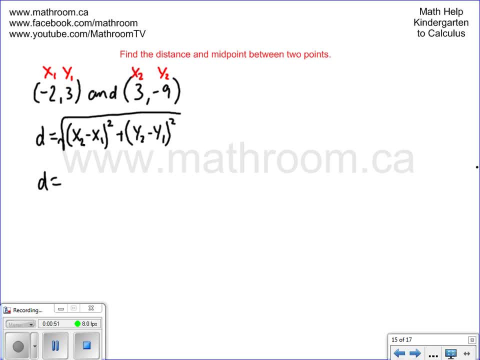 formula: Distance equals x2 is 3 minus a minus 2,, which is x2.. So we have x1 squared plus y2, which is minus 9, minus y1, which is 3 squared. and we're going to take the square root of that: 3 minus minus 2 is 5.. So we have 5 squared plus minus. 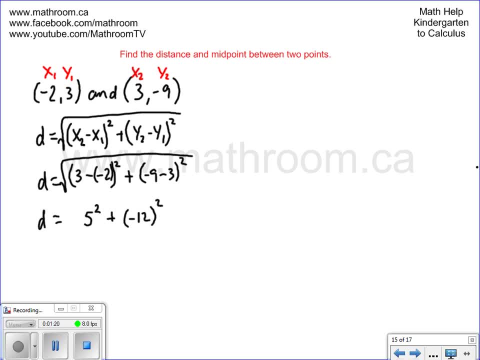 9 minus 3 is minus 12 squared, 5 squared is 25.. minus 12 squared is 144,. 25 plus 144 is 169, and the square root of 169, distance, equals 13.. So the distance between minus 2, 3, and 3 minus 9 is 13 units. Now how do we find? 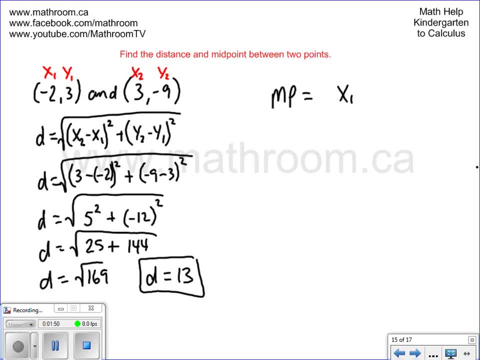 the midpoint. Midpoint equals x1 plus x2 divided by 2, and y1 plus y2 divided by 2.. And that will be obviously a point We plug in the values. x1 is minus 2, plus x2 is 3.